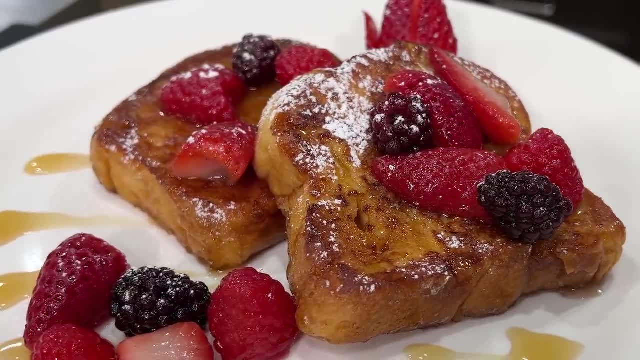 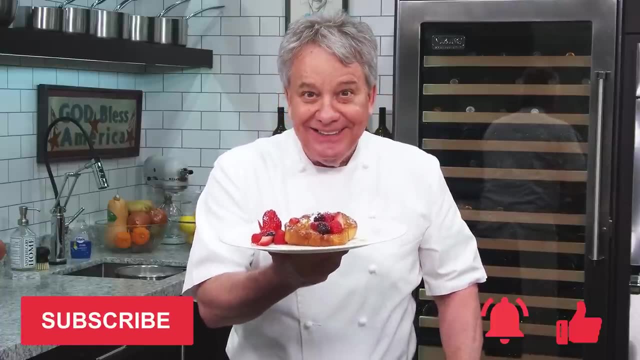 Hello there, friends. Today I'm making french toast and I'm using brioche bread. Remember, thumbs up. if you like the videos, subscribe to the channel and ring that bell. Stay tuned, we're gonna do it right now. Well, hello there, friends. Let me show you how to make this. This is really a beautiful. 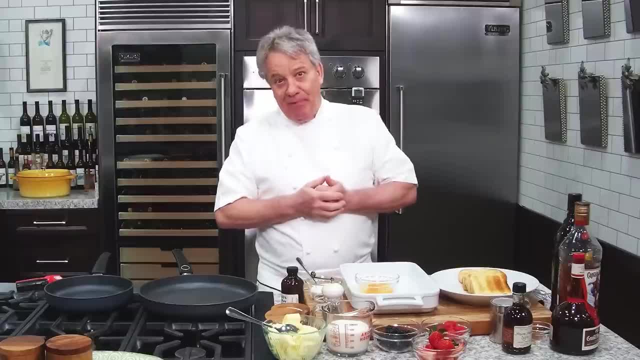 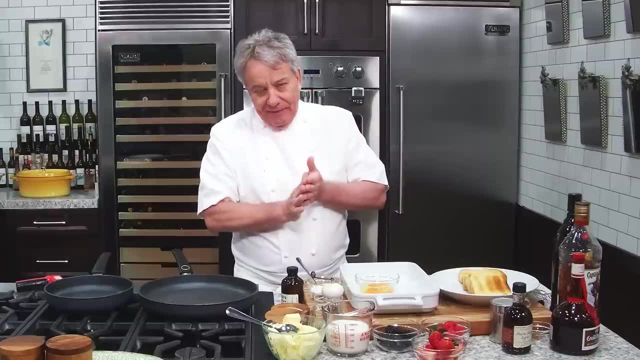 recipe Very simple to make. You know I like brioche bread, so I'm gonna use the brioche bread To make a french toast. you have to have thick bread, So you get a brioche bread, you slice it. 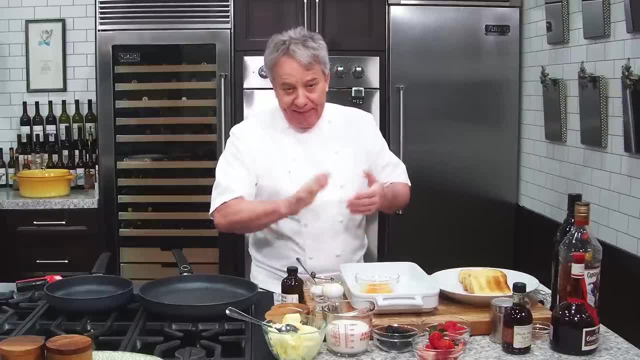 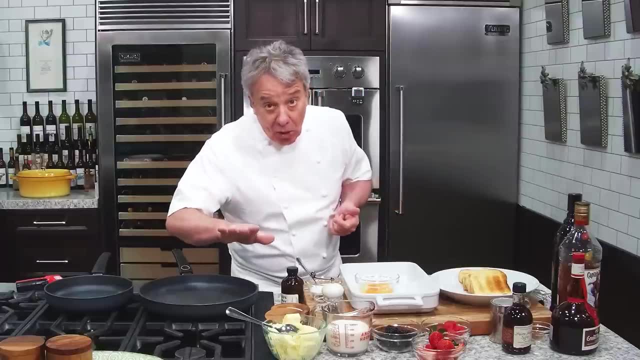 or you can get whatever bread you want. You know so. so good is raisin bread. Anyway, in french it's called pain perdu, Pain perdu, which means lost bread. Usually you make it with the old bread. I don't like the old bread, Gold bread, I give it to the duck. But make it with whatever you want, Whatever. 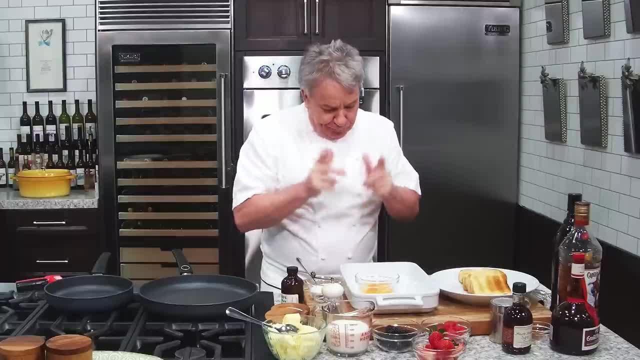 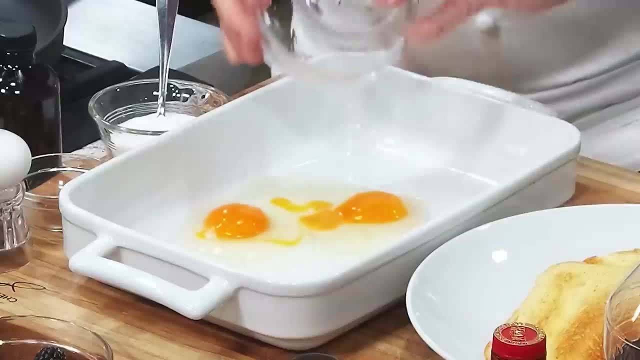 bread you want is okay too, All right, um, what we're gonna do, we're gonna make a batter. A batter, We're gonna put the eggs and, uh, and let me just do them, Let me just put them in right in there, right, Eggs? 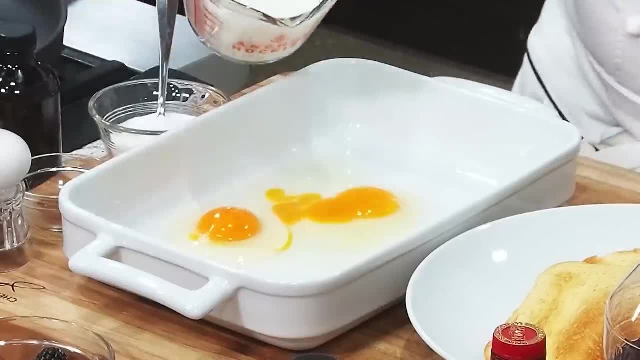 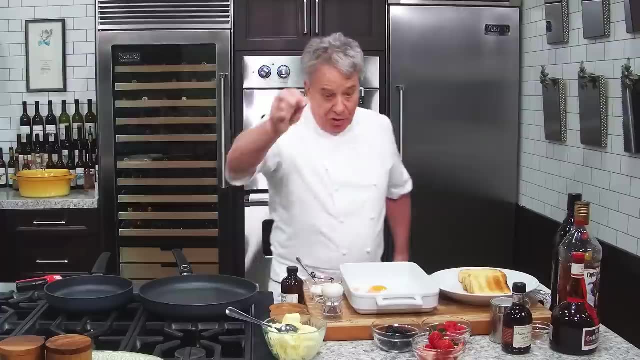 and then we're gonna make a brioche bread. We're gonna put a little bit of milk about, like maybe a quarter cup of milk or something like that. I'm not really measuring carefully, but you get an idea right. A pinch of salt, Always put a pinch of. 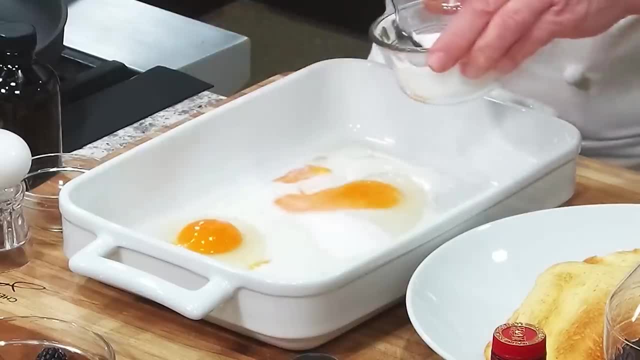 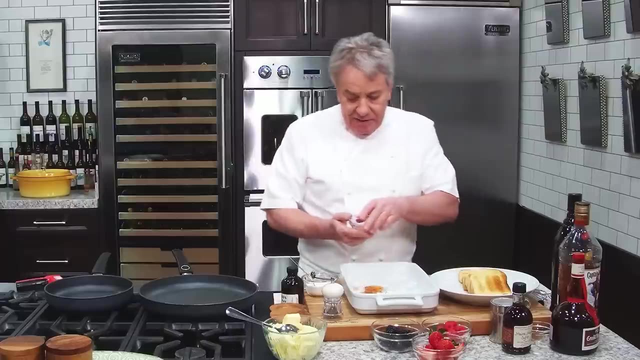 salt. It doesn't matter if it's sweet or not. We're gonna put a little bit of sugar, Measure everything carefully. A little bit of cinnamon, Cinnamon friends. I love it in the background, not in the foreground, Like I don't want all of a sudden: oh Now some people like cinnamon. then 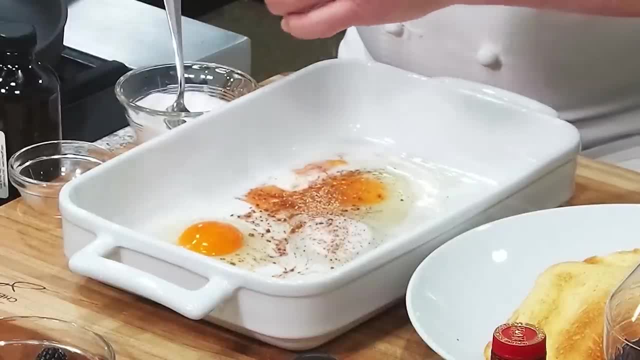 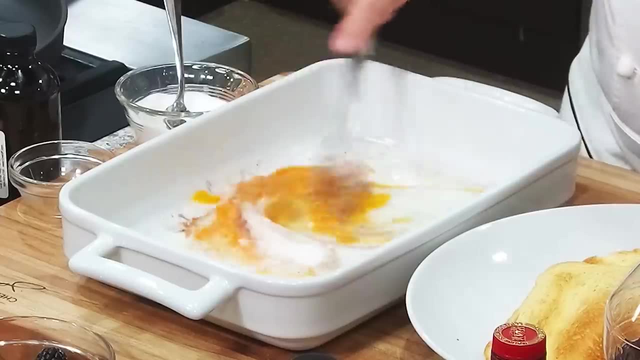 put away. however, you want A little bit of nutmeg, Ground nutmeg. I got this nutmeg grinder. It's pretty cool, but you can use just a pot of nutmeg, right? And then what we're gonna do, It's really simple. I mean, a child could do this. 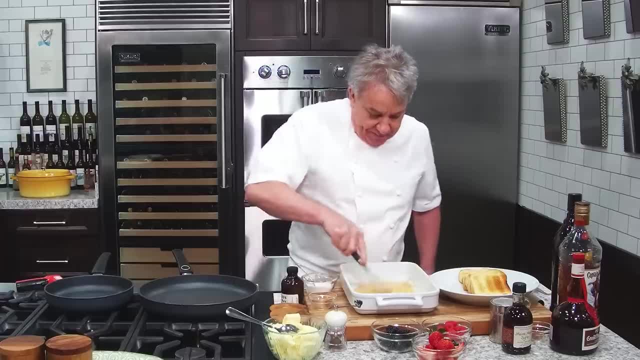 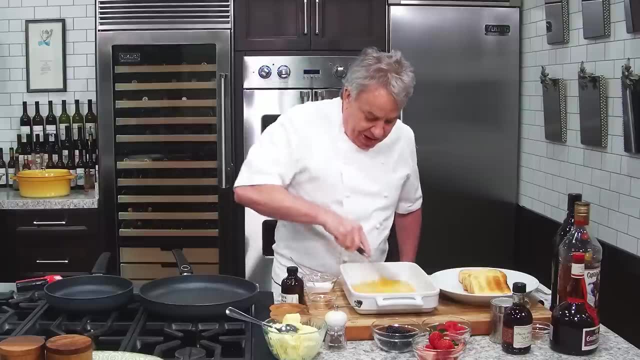 I know if you said oh yeah, oh come, your eggs are so yellow. It's the uh um free range eggs that I get at the grocery store. I we get them at Publix. They're wonderful. Maybe just a little bit more milk, What do you think? Just a touch more milk? See, that's the whole idea about. 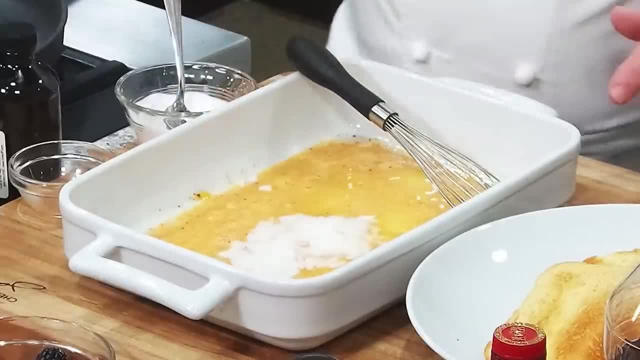 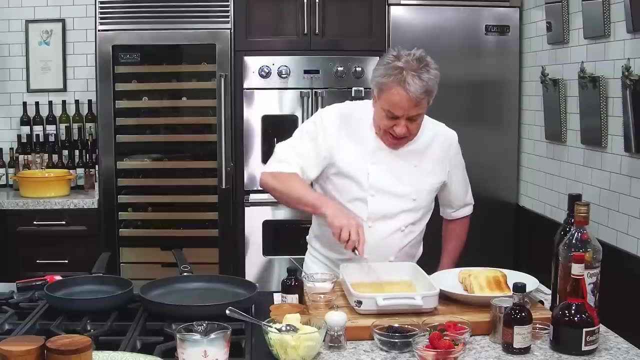 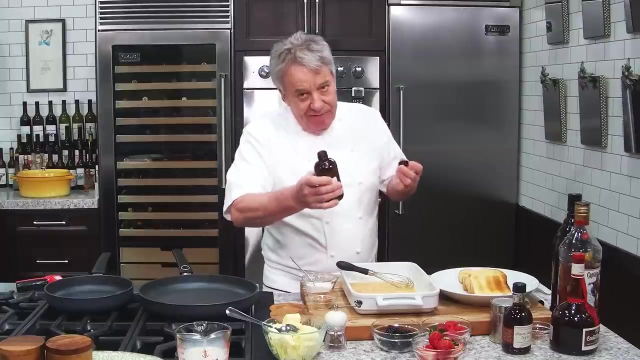 um is uh uh percentages, just doing it. however, you want quarter cup, here you go. i got enough right there and you know what i like to do. also, i got to put some tahitian vanilla. i like to put uh uh tahitian vanilla. you can get whatever vanilla you want. i think tahitian vanilla is one of the most flavorful. 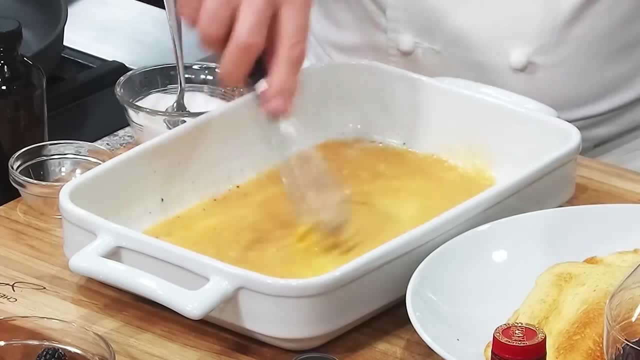 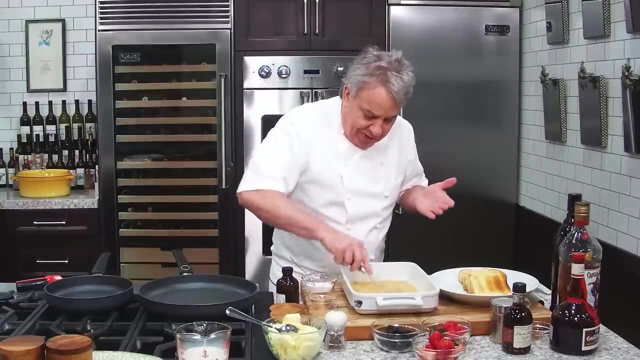 vanilla, but uh, madagascar vanilla, mexican vanilla. there's a lot of vanilla out there. if you can get pure vanilla, it's better, but if you can't, you can't. you know that's it. i'm gonna put just a touch more milk. you see, where is it? where's the milk? hope, here it is. 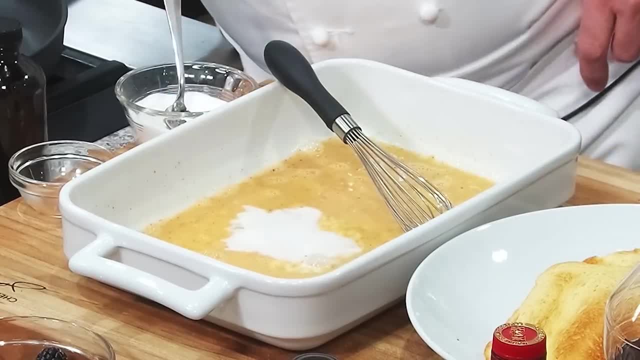 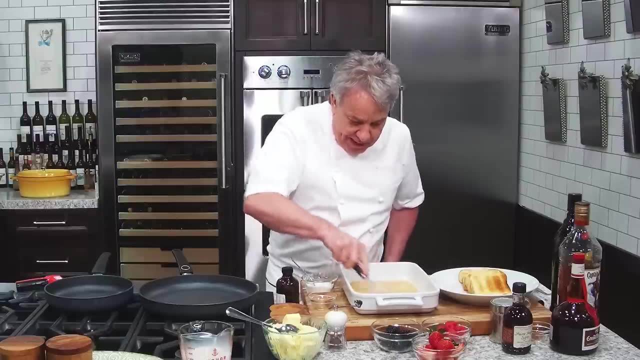 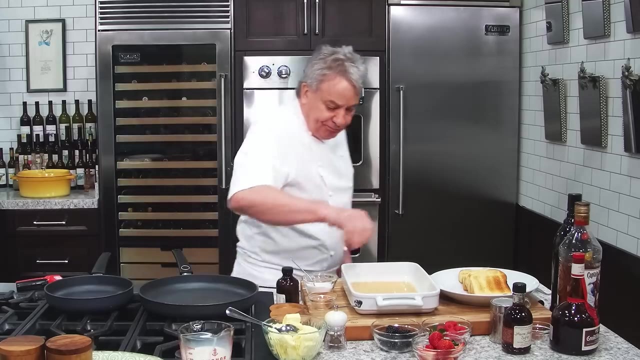 and i knew people in the channels here: this guy's nuts and that's okay, we don't mind having this label. so now, what else did i do to this? okay, i got it more ready to go right. very simple so far. let me move stuff out of the way. this i'm gonna need later. 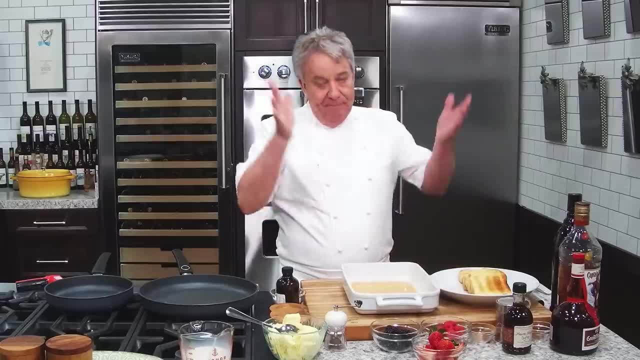 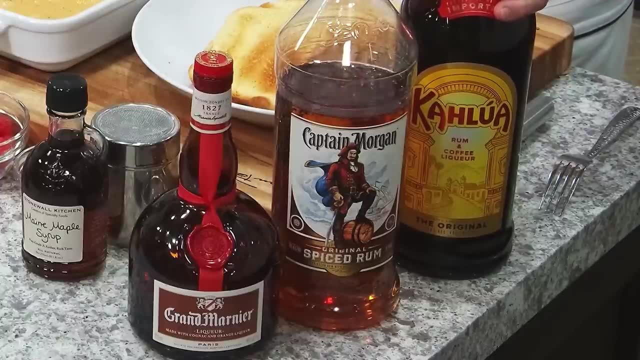 this. i don't need what else that we're gonna put in here now the adult version: little bit of calor, a little bit of rum, and you see, i got grandma. and yes, because i'm gonna put some berries, i'm gonna saute them in a simple syrup with a little bit of butter in there. 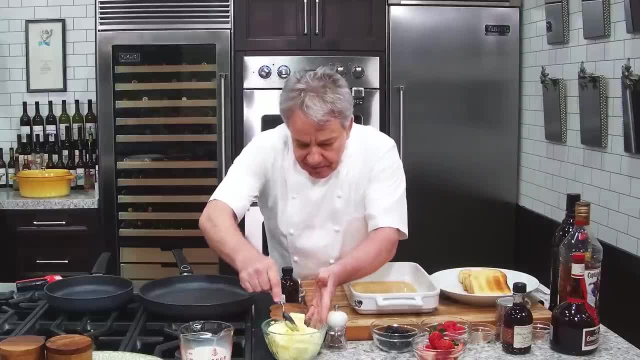 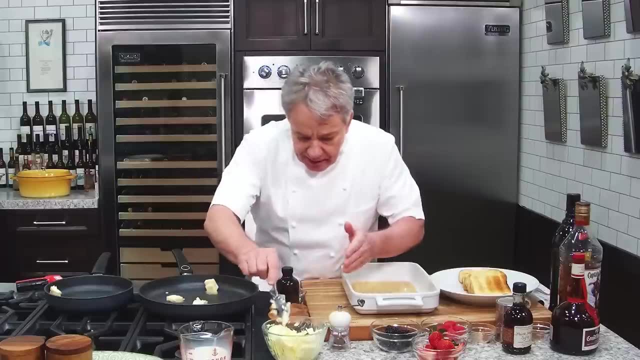 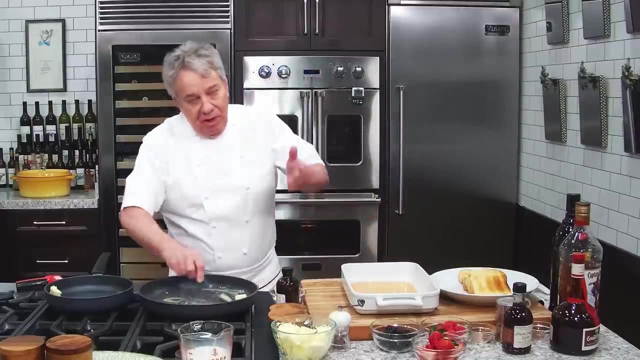 and uh. so oh, by the way, talking about butter, let's get ready with our butter friends. we're gonna put a little butter. we're gonna put some in here too. we're gonna use that later. a little butter, real butter, yeah, like you can't really have too much butter, right? i mean, we all know that. 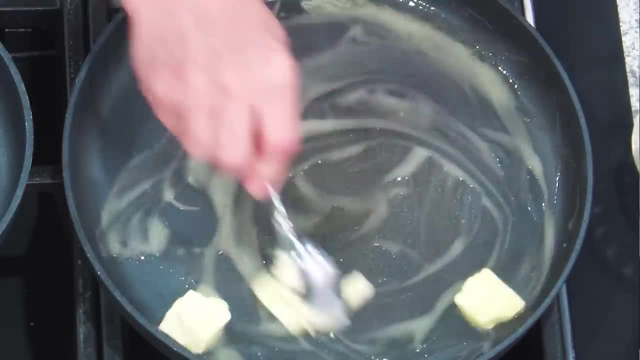 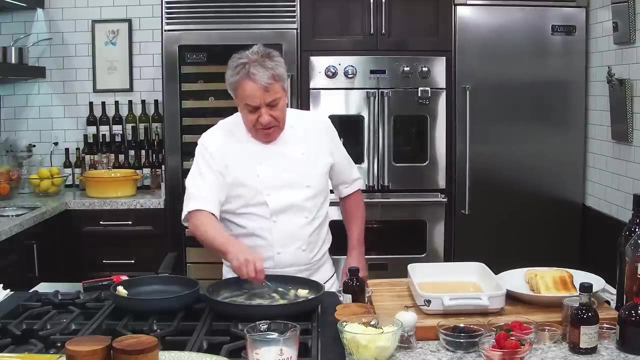 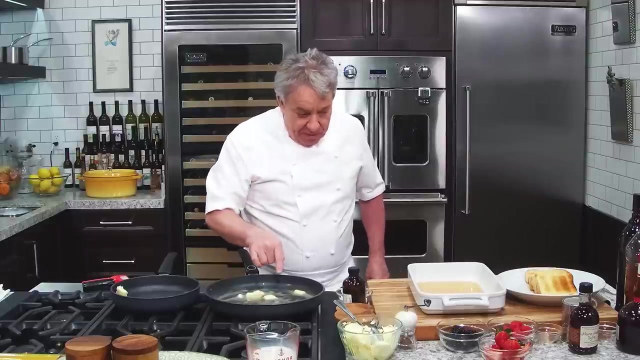 butter is good for you. i mean, i always push butter and people said, oh, you use too much butter. what do you think? not too bad, right for a guy who eats a lot of power? i eat probably a quarter pound of butter a day. that's a lean day for me, uh. so we're gonna put that in there and 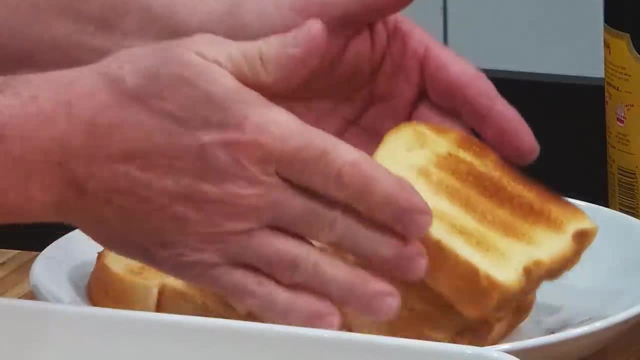 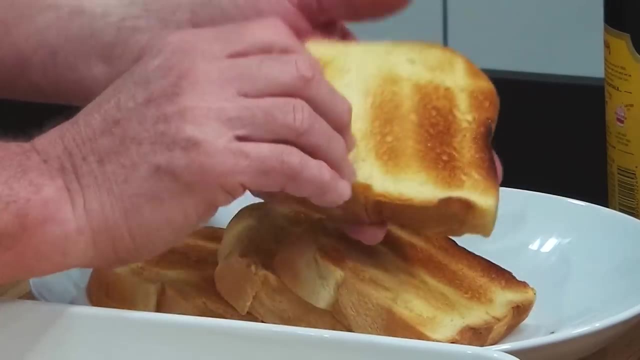 we're gonna put the bread. let me tell you about the bread. friends, it doesn't matter what bread you're using. if you're using a brioche bread, you're using a brioche bread, you're using a brioche bread or whatever favorite bread you use. i like to toast them and i like to uh, and the reason why in. 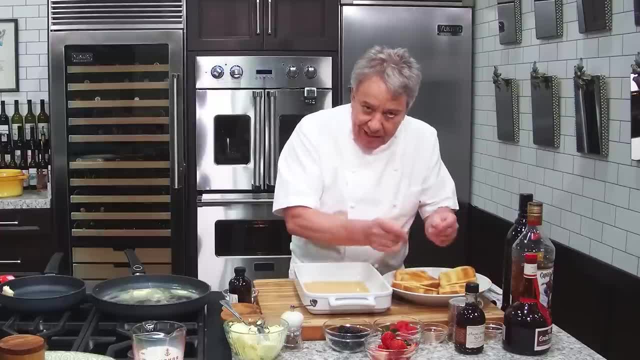 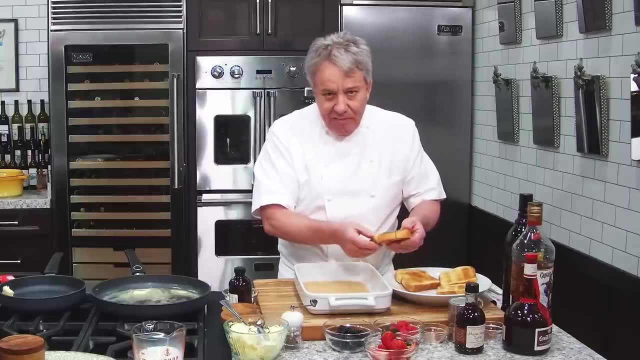 france they use the, the old bread, is because we kind of like a little dry. i don't like a dry really, so what i do is i toast them. they still tend to in the center, but what happened is the fact that they are a little, uh, crusty on the outside. they're not gonna get soggy, so it's. 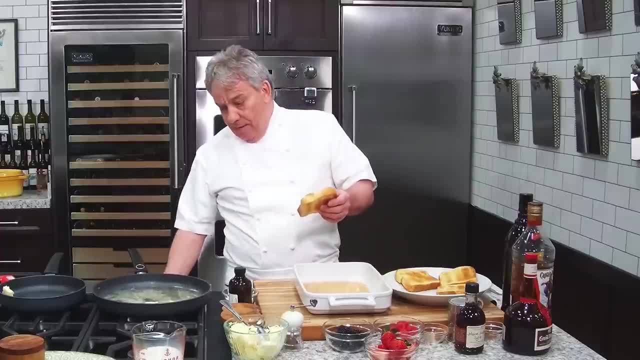 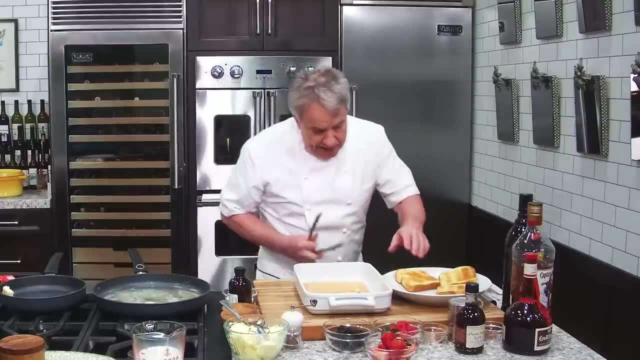 really an important little thing to remember, my friends. okay, you want to toast your bread first, it doesn't matter what bread you're using, we're going to keep it. we're going to get them in the um, in the butter than we made, but we're not going to leave in there and they're too long, just. 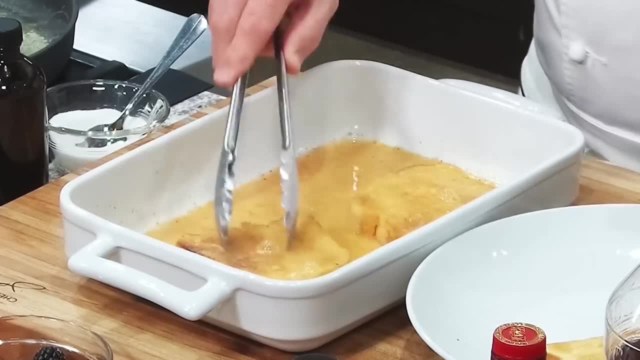 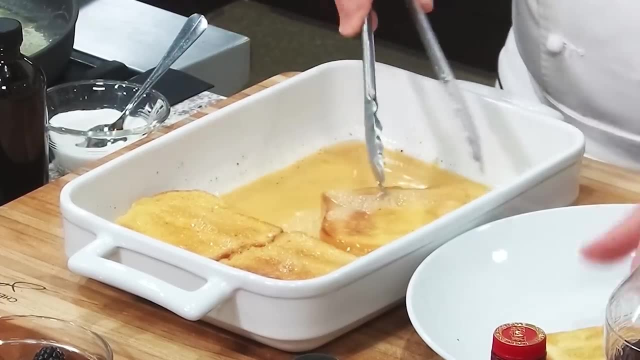 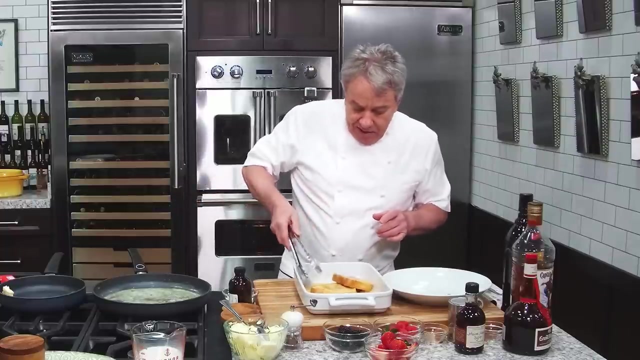 a few seconds on each side. we don't want them to get soggy, okay. so we're leaving in there a little bit, just for a few seconds on each side, you see, and then we're going to put it in. this is really simple, friends, i mean really french toast, i mean really. okay, everybody's been asking me: please give. 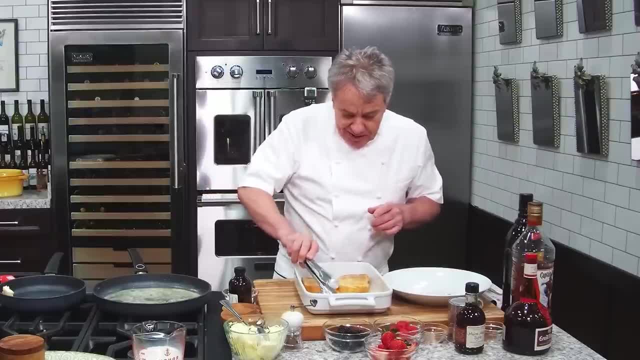 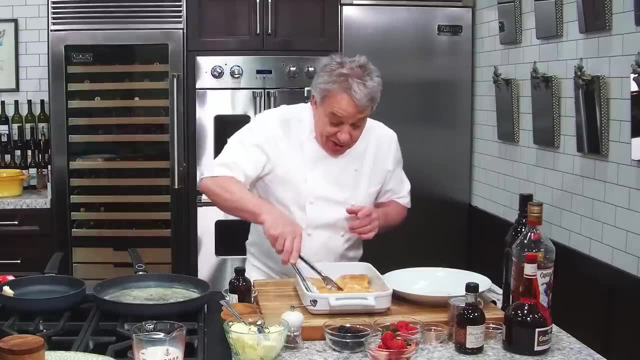 it a try, all right. so this right there, and then i'm going to do these, uh, berries, see, all right. so what do you think i think that's, what do you think i love? when i ask you all the time, what do you think you know? it's because you know. remember, when i had the cooking school, every night i would cook. 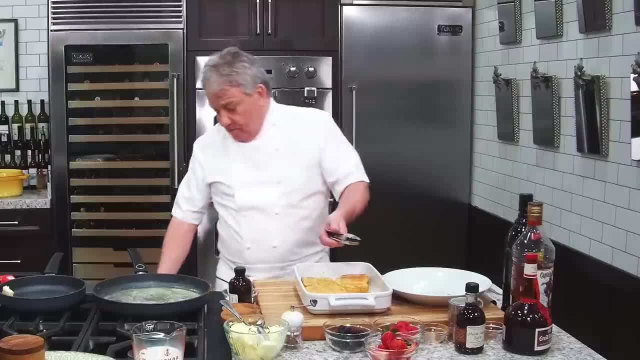 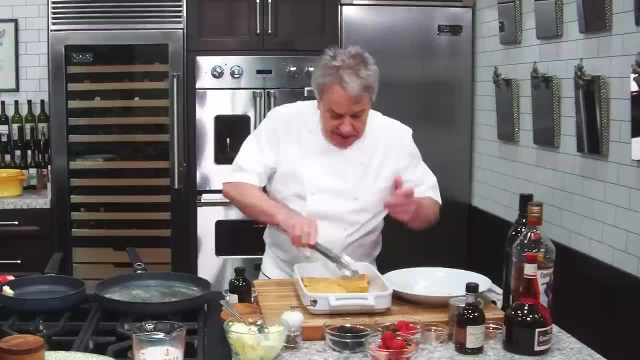 every day i would cook in front of people and they were right there in front of me. i had to ask them what they thought, because they were going to eat everything i was going to cook, all right, they were going to eat it all. so i had to ask them. so i'm keep asking you. 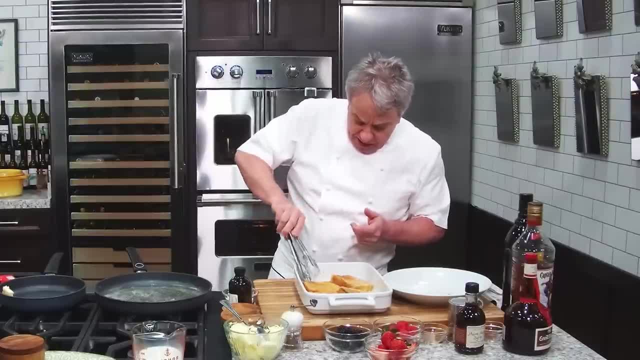 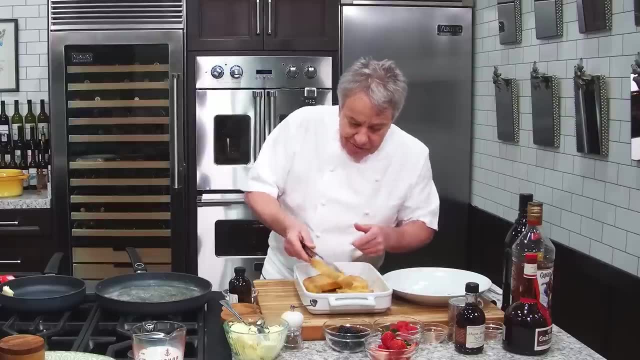 i hope i put everything in there that i was supposed to put. see, look, i drank the whole thing and they're not going to get soggy. they're not going to be soggy because, uh, that dish was a little smaller. they're not going to get soggy because, um, you know, butter should be a little. 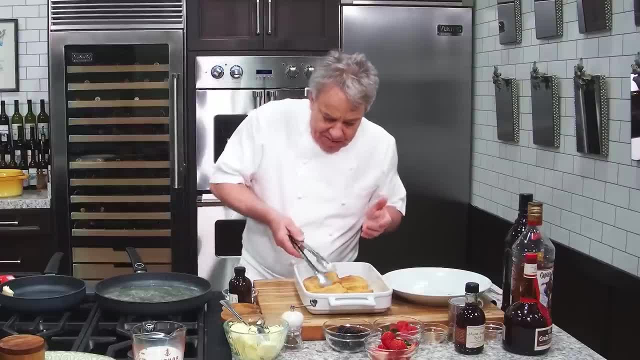 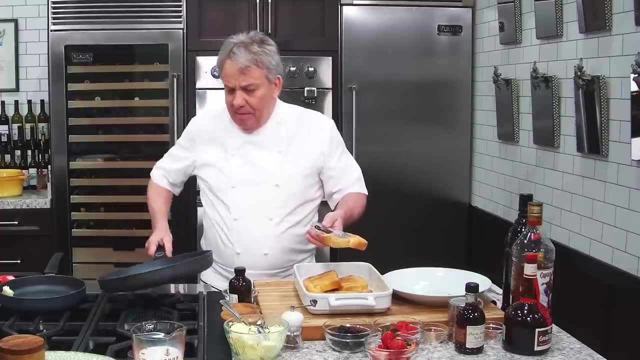 harder. they're not going to get soggy because we took the time to toast them before, okay, so it's really really important. make sure your butter is a little hotter than mine right there. that's always the problem when we're doing live things, live shows. let me take it out of here because 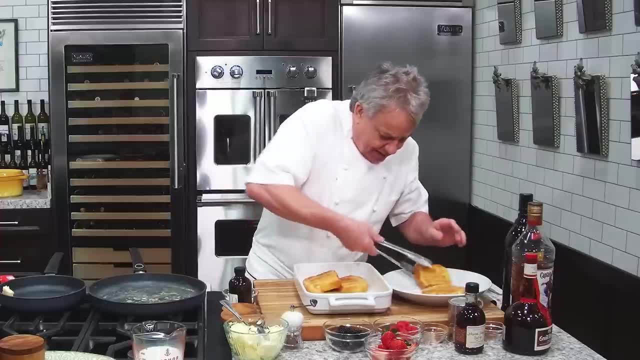 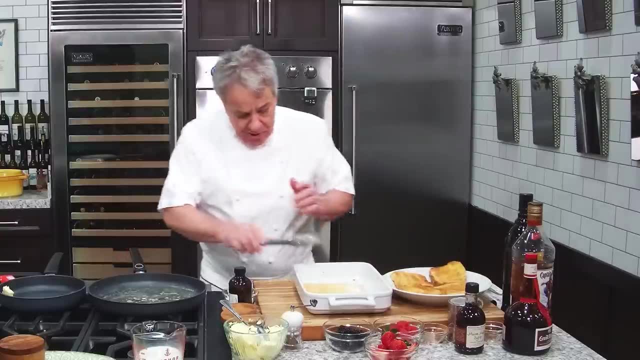 i don't want it to get too soggy. i don't want it to be soggy, okay. i want them to be soft, but not soggy, all right. so let's make sure this is hot. let me get a rag. i wanted to be outside. you know they're gonna be beautiful. you watch, this is gonna be delicious. 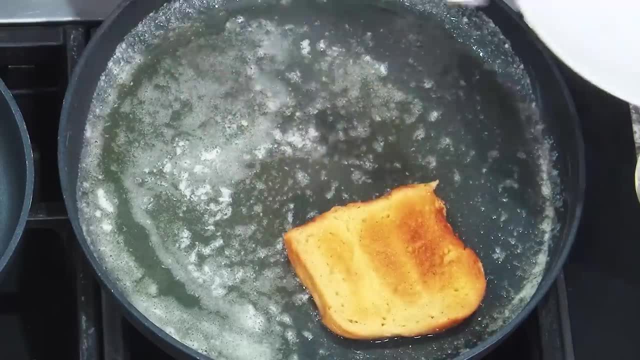 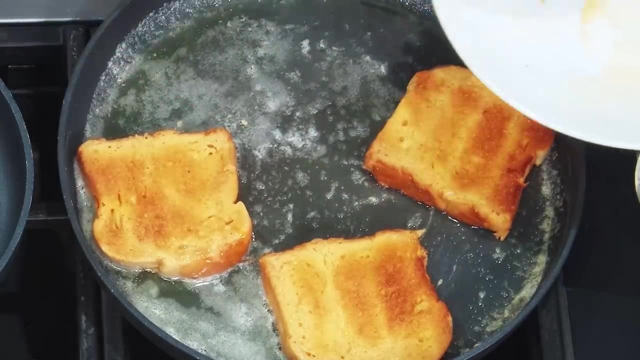 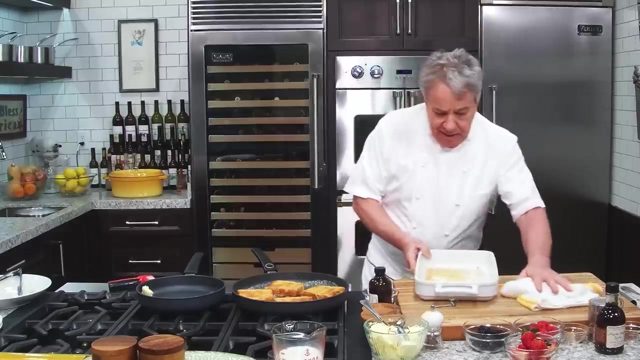 my friend: all right, so here we go, put the bread in here. yep, there you go. they should fit in that pan pretty good. and then we leave them alone for a second. okay, while they are getting nice and and golden brown, let me remove all the stuff i don't need out of here, friends. 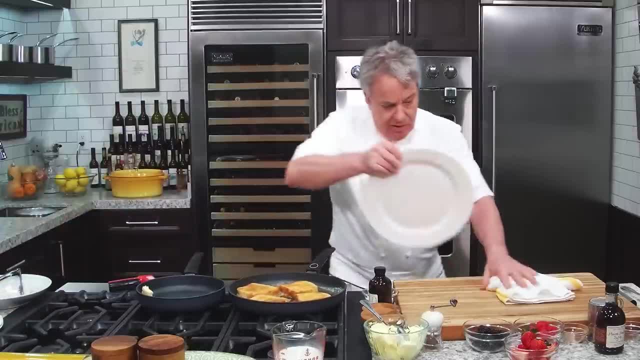 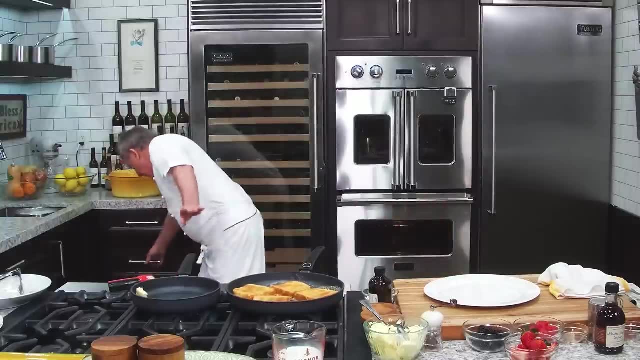 when they're getting nice and golden brown. i got a plate right here that i'm gonna use. let me now take care of the fruits and the fruit. oh, you know what? i gotta get a spatula. i forgot to get a spatula, but i got it. i got everything. that's the cool thing about this. 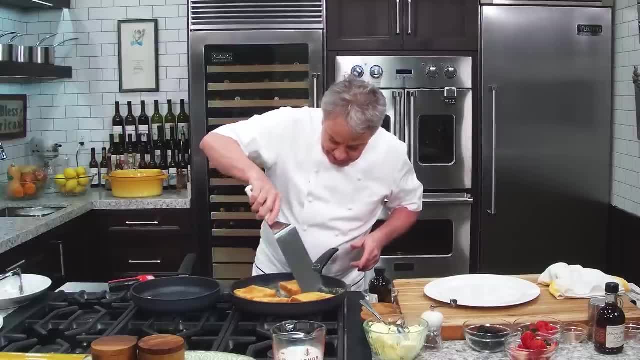 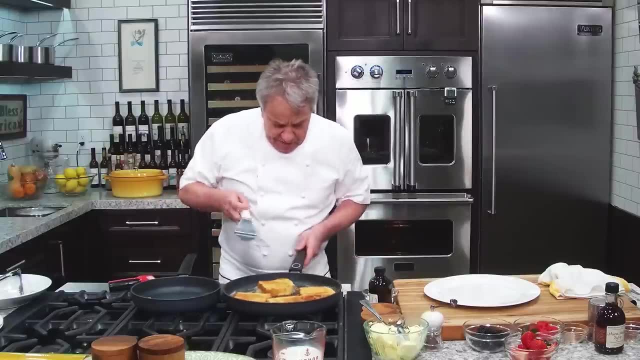 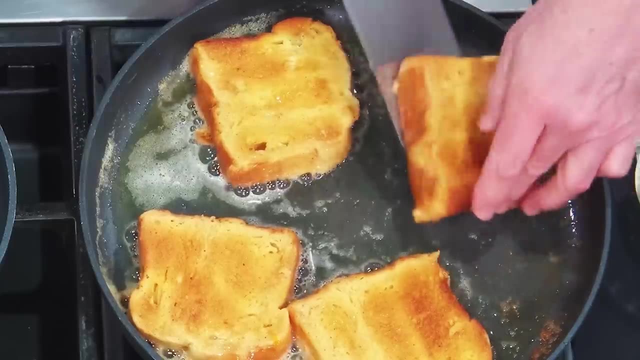 kitchen, friends, i have everything. well, guess what, after 50 years in the kitchen, you should have everything right. we want them to be beautiful, golden brown, not too cold and brown, but we want them to be pretty enough. so let's make sure the butter is not too hot. all right, let's see what we got here, friends, they're not there yet. all right, okay. 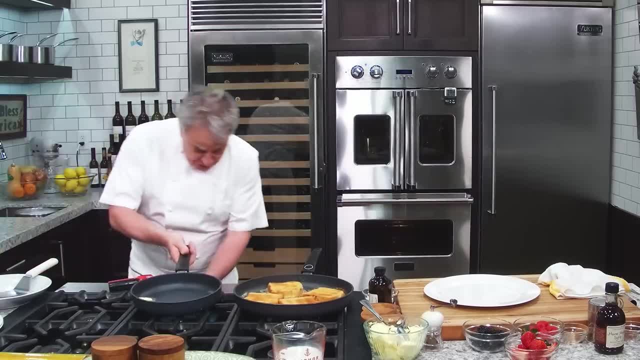 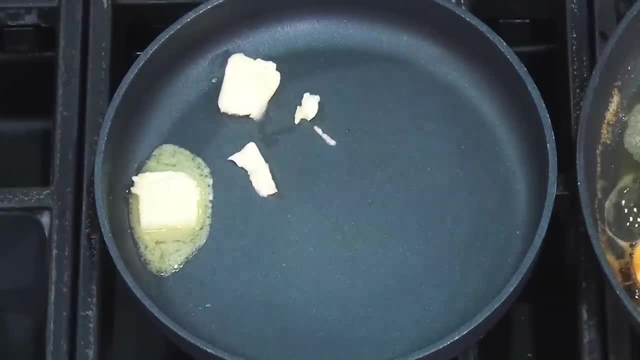 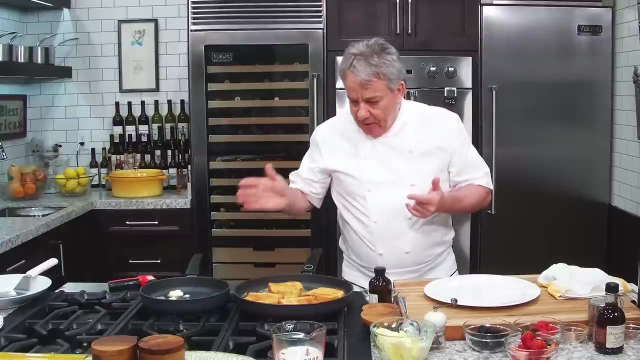 that's good. that's good because we've got a few minutes. we're going to do the fruits and the fruits. all i'm doing is putting in a little butter. now you know what? the adult version, the rum and the color go right ahead, don't be afraid to do it. and the adult version for the. 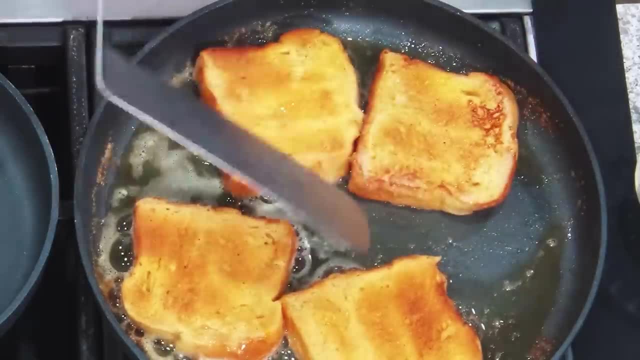 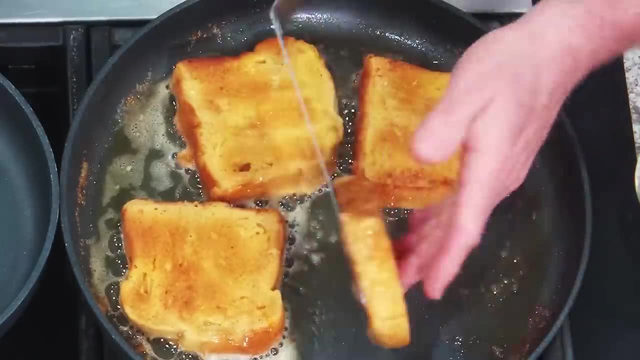 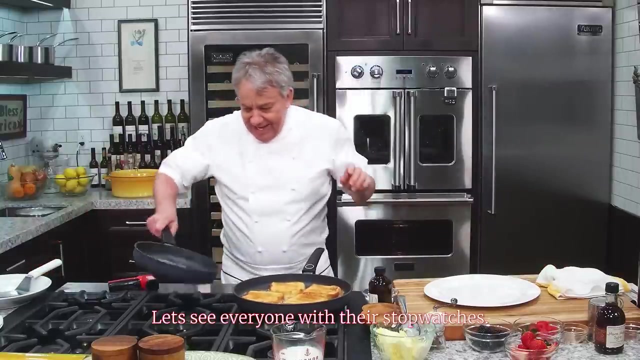 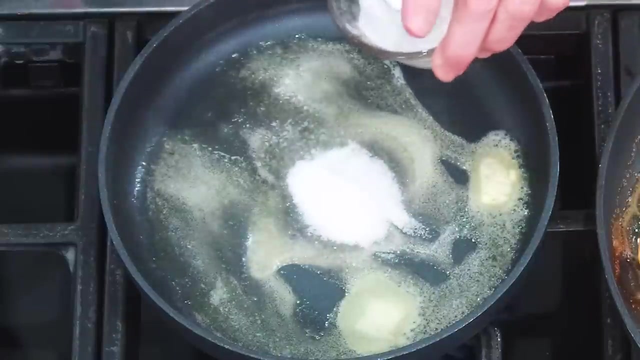 oh, let me make sure this is. and I yet now, yet, well, now that I flipped it, let me see, because it smells, not yet another 12 seconds, something like that. the, the, the adult version for the fruits, I mean funny, obviously for the kids. you just put butter and sugar and you put it on water so you get like a simple syrup, the. 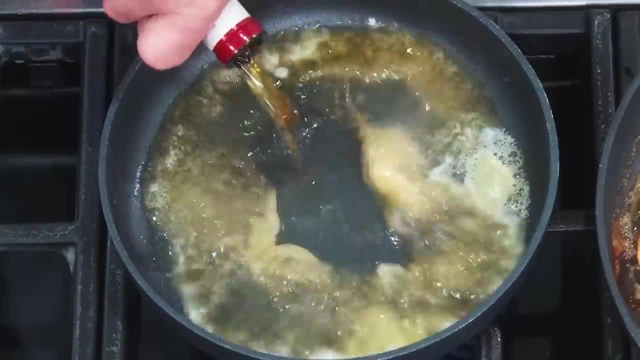 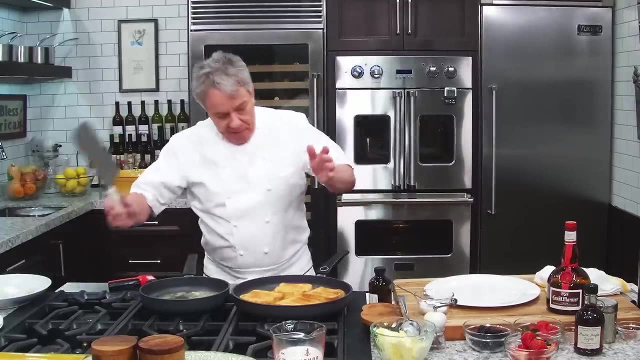 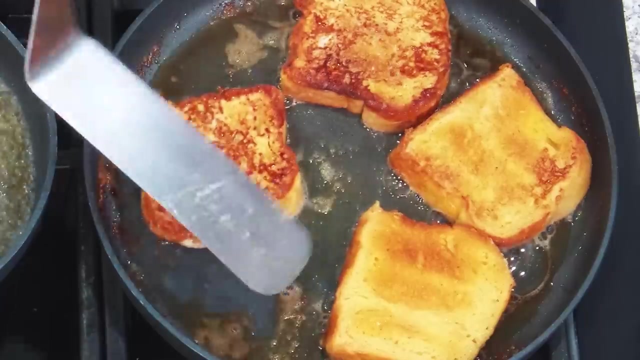 adult version. you put it on grandma in there. that's the adult version. orange juice for the kids, always just for a kid. it'd be perfectly fine for the adults. yeah, now we're talking. look, look, you see, it's what I want. this is what I want to. 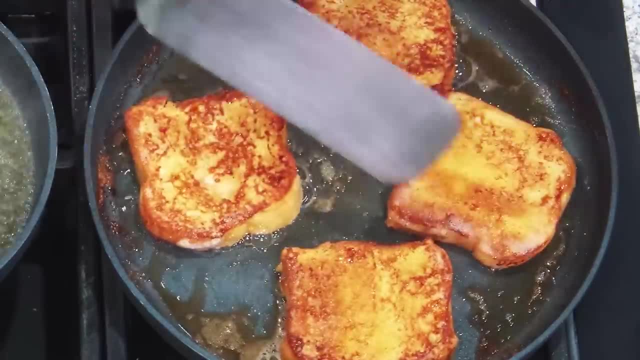 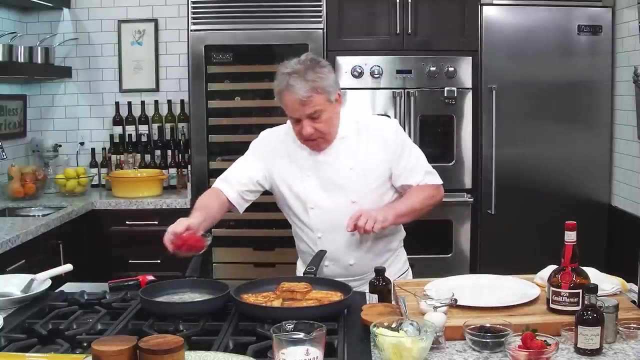 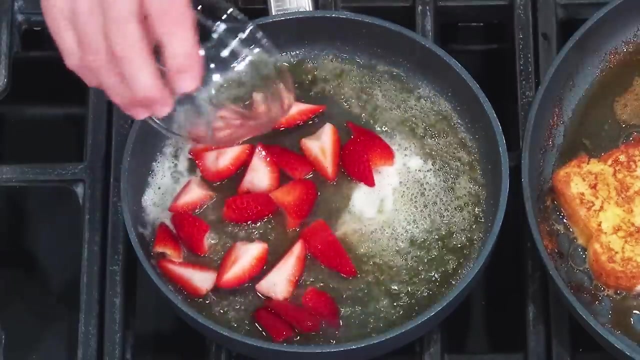 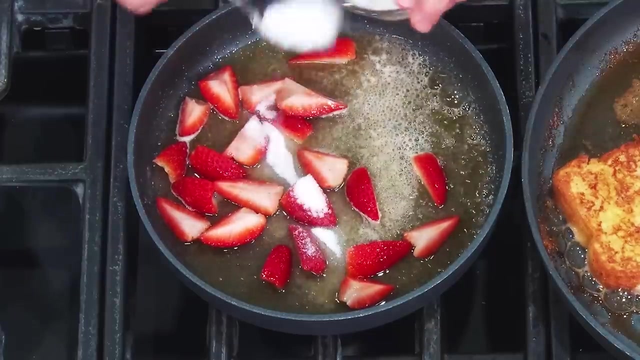 press. look at this. oh yeah, baby, look at this. all right, so the fruits: I got raspberries, I got blackberries and I got strawberries- strawberries, we're gonna put them first because the strawberries could cook a little bit. the other one, I don't need to cook at all. put a little more sugar. I like it to be a little thicker, right? 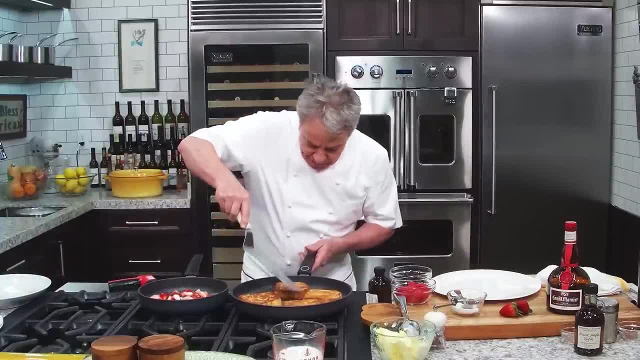 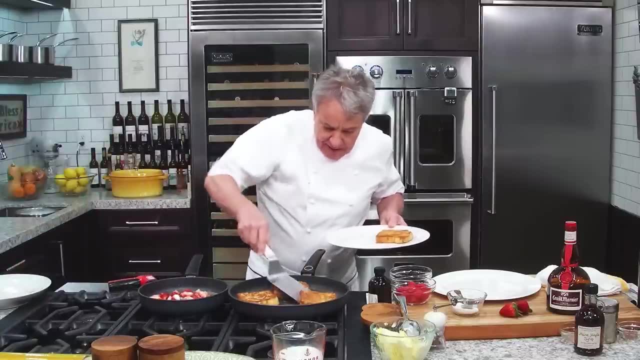 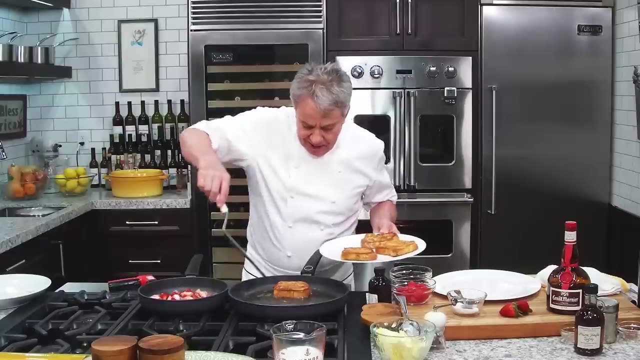 let's take the, the French toast, out of there. let me put them in a plate here, and then I, in a minute, I'll make a nice plate for serving. we're gonna keep them so they don't burn on us. you see, that's exactly the way I like it: nice and golden brown, like this, beautiful. let. 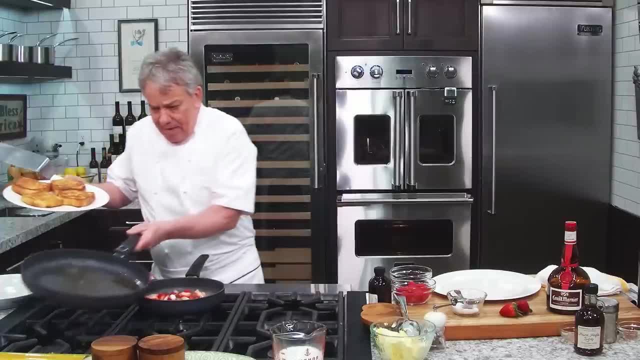 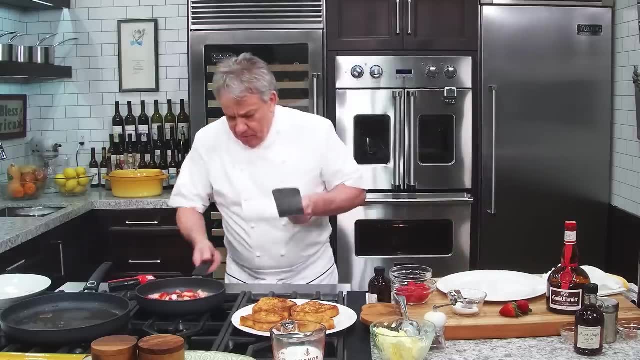 me turn this off. I never have the room there. you go. you know I'm gonna keep it right here. oh, it's gonna be at the plate, gonna be hot down here. don't grab the plate, all right. so here's what we're gonna do. we're gonna saute a little bit. 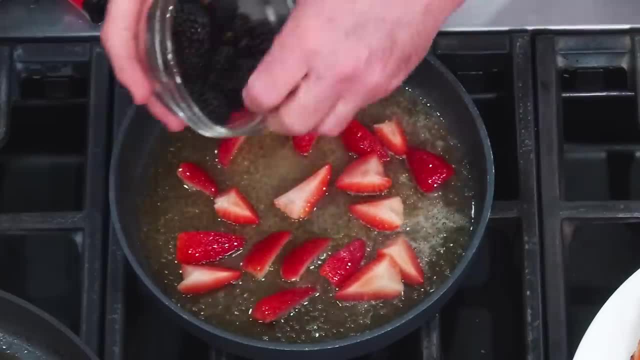 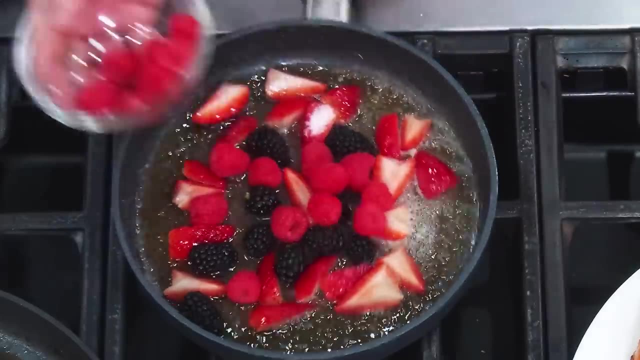 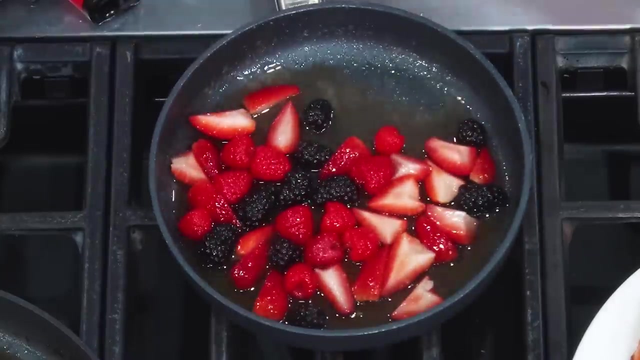 of fruit right there. we're gonna take the blackberries- they don't need a cook, just get them a little thing. and especially the raspberry, they don't need a cook, we just got to get them coated. or we trying to do is just get them coated. we let them cook for a second, so we take. 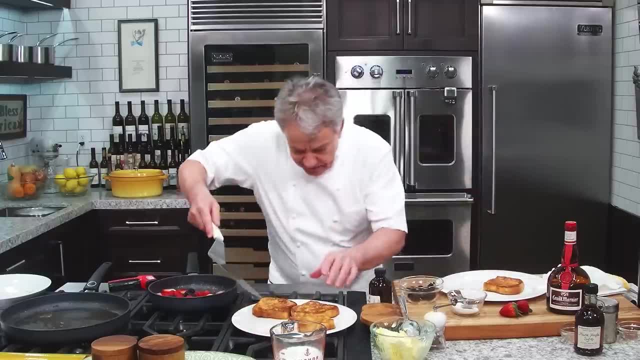 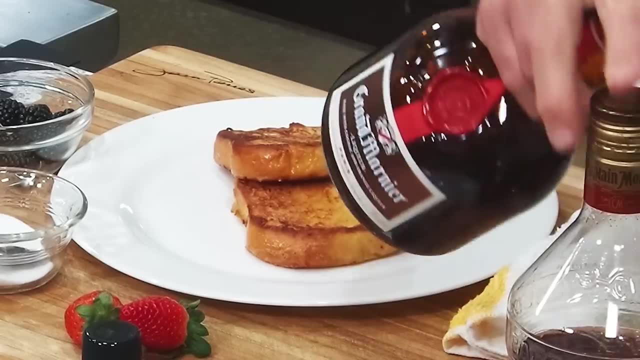 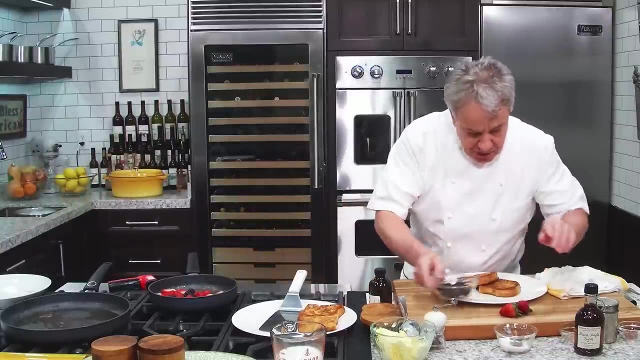 our slices right there. oh yeah, this is gonna be delicious friends. right, take a plate right there. let me tell, let me remove this out of the way, for so the camera I can see because I always have things in the middle. all right, so we're gonna decorate with a, with a raspberry, then we're gonna take a little bit of the. 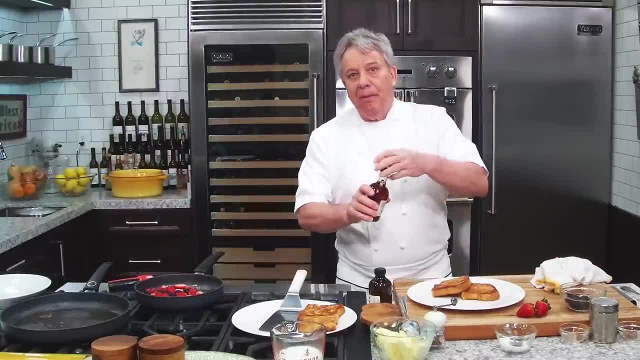 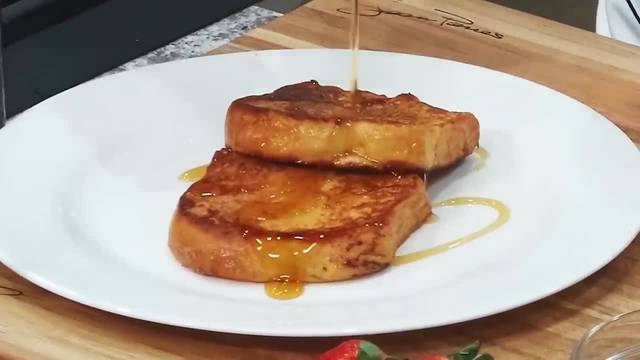 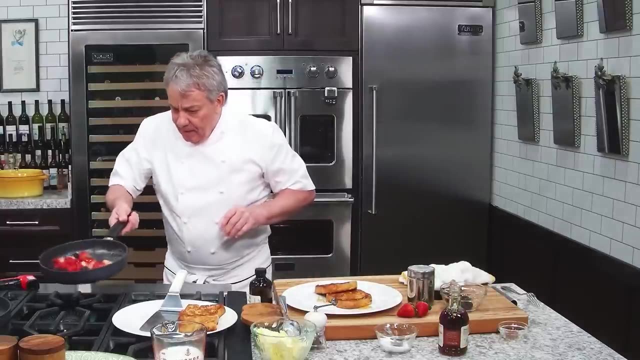 maple syrup. I love a little maple syrup on it. you don't have to put maple syrup, you can put whatever syrup makes you happy. just a little bit on it. oh yeah, mm-hmm, yeah, little maple syrup. what is? a little bit of fruit, just a little bit of. 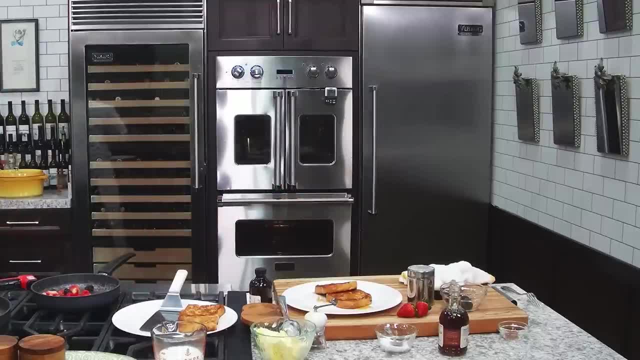 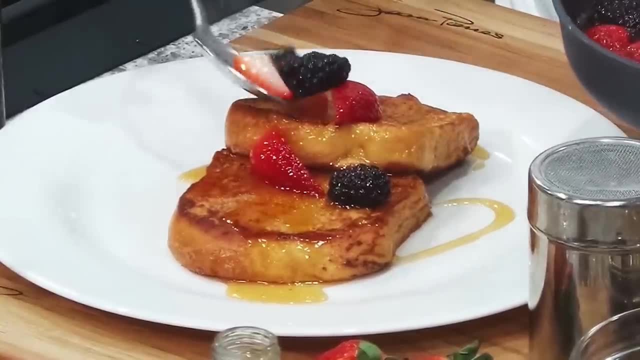 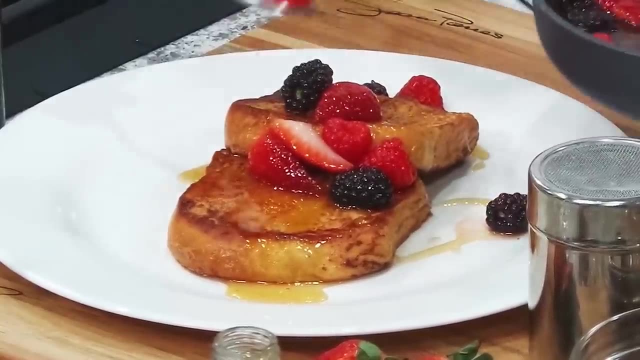 fruits: one, two, three. let me get a spoon. I mean, this is so simple, my friends, take a little bit of the fruits right there. oh yeah, you can put more syrup if you want. it's really up to you. this is beautiful, simple child could do it. that should be.